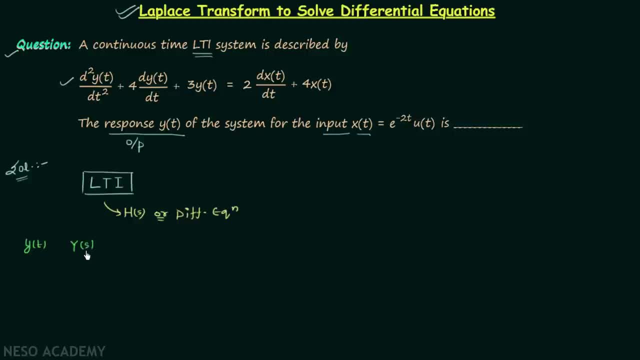 we know it's Laplace transform ys. because if we know ys we can perform the inverse Laplace transform to obtain yt. and we can have ys if we know the transfer function hs, and the Laplace transform of input xt, because when we multiply hs and xs this will give us ys, because we know 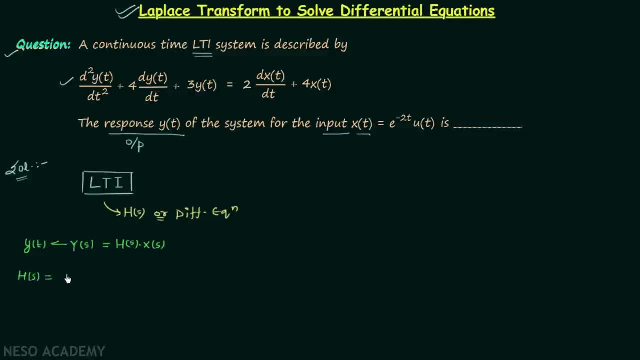 the transfer function, hs is equal to the Laplace transform of the output, which is ys, divided by the Laplace transform of the input, which is xs. and while defining this, we consider all the initial conditions to be zero. Now here, if we know hs and xs, we can multiply them to get ys. and once we 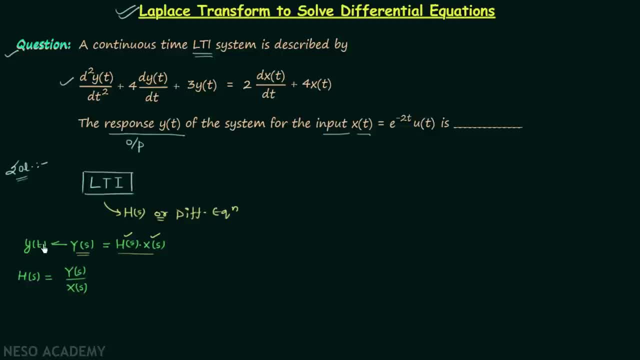 have ys, we will perform the inverse Laplace transform to get yt. So we will focus on calculation of hs and calculation of xs. We can easily calculate xs because xt is given. The only thing we need to do is to obtain the Laplace transform of this time. 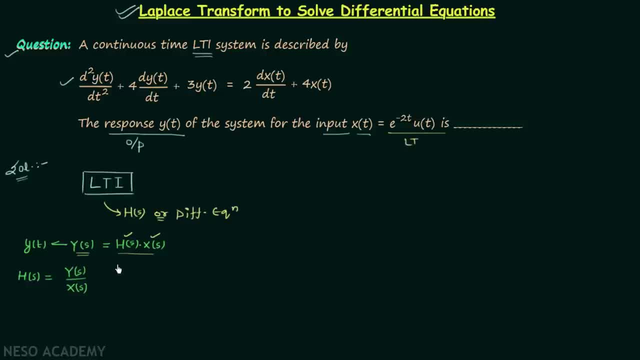 domain signal. It will give us xs and to obtain hs we will perform the Laplace transform on the given differential equation. and this is our main concern. We are understanding how to solve the differential equation, So let's move towards the solution of the question. I will first write down the given 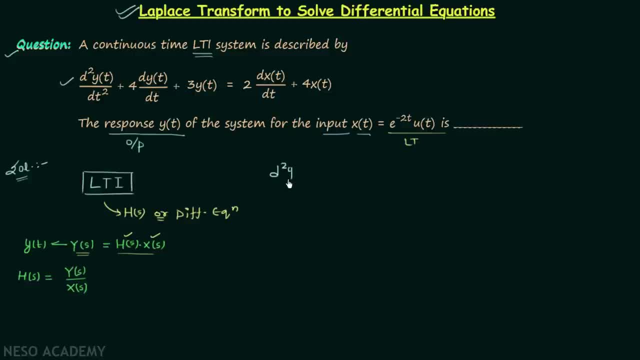 differential equation. It is 2 times derivative of the output yt with respect to time t, plus 4 times derivative of output yt plus 3 multiplied to the output yt. and this is equal to the 2 times derivative of input xt, dxt over dt, plus 4 times input xt. Now to obtain the Laplace transform: 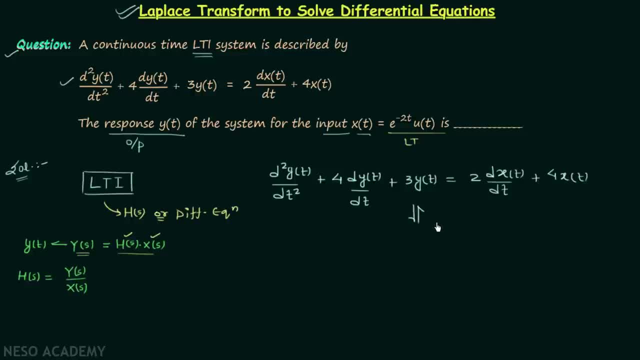 of this differential equation, we are going to use the differentiation in time property of Laplace transform. So let's quickly revise the differentiation in time property. If we have a time domain signal ft, and this signal is having the Laplace transform equal to fs, and we are talking: 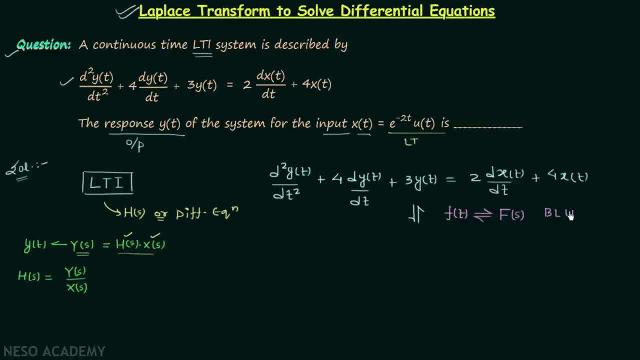 about the bilateral Laplace transform. Now, if you differentiate the time domain signal ft n times with respect to time t, then the corresponding Laplace transform of this time domain signal will be s power n. So we are going to use this property and let's say output yt is having the Laplace transform. 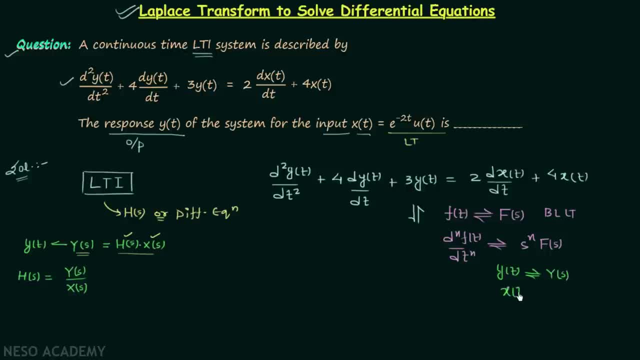 equal to ys and the input xt is, having the Laplace transform, equal to xs. So let's move to our next step. We will first focus on this term, the 2 times derivative of yt with respect to t. Now compare this with this: you will find n is equal to 2.. 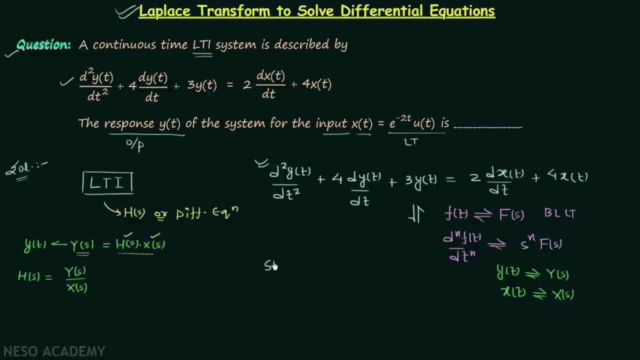 So this will have the Laplace addicted to. you can see we are having s power n. So, replacing n by 2, we will have s power 2 multiplied to the Laplace transform of the output yt, which is ys. Similarly, we will have 4 multiplied to s multiplied to ys plus 3. 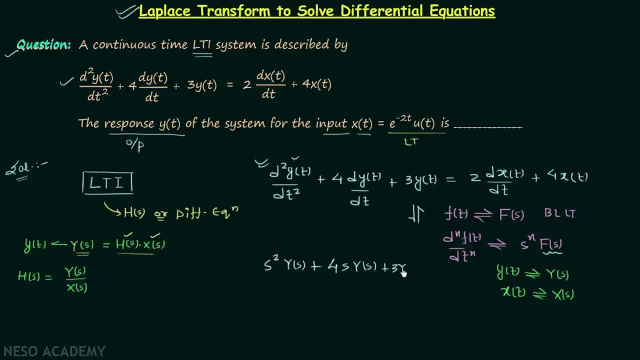 multiplied to 7.. Now compare this with this: You will find n is equal to 2.. So this will have the Laplace plus 3 multiplied to ys, because here we are only having yt multiplied by 3.. There is no derivative of. 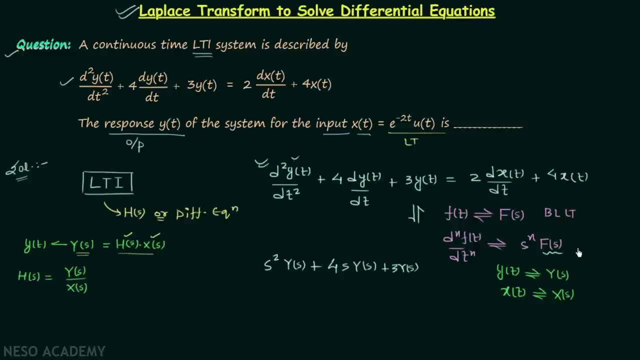 yt, so there is no need to use this result. We will directly write down 3ys, and on the right hand side we will have two times s multiplied to xs, and as we are not having more space here, I will write down the Laplace transform. 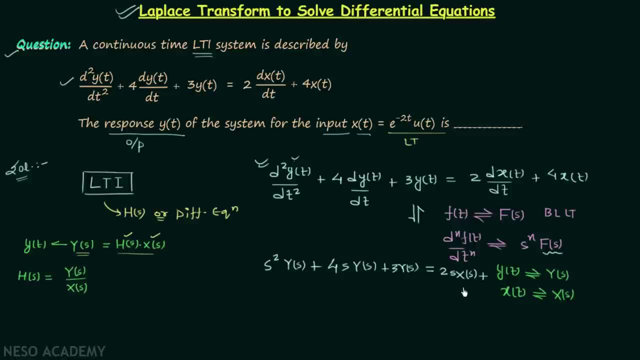 of 4xt. here The Laplace transform of 4xt is equal to 4 multiplied to xs. So this is what we are having as the Laplace transform of the differential equation, and on the left hand side I will take ys common. so we will have: 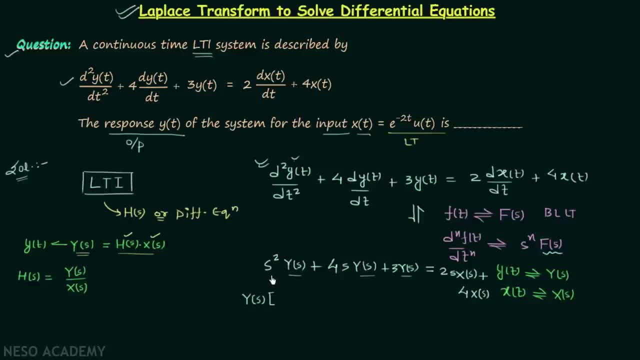 ys inside the bracket s square plus 4s plus 3, and on the right hand side I will take xs common. so we have xs inside the bracket, 2s plus 4 and we are looking for the transfer function of the LTI system and the transfer function is equal to ys. 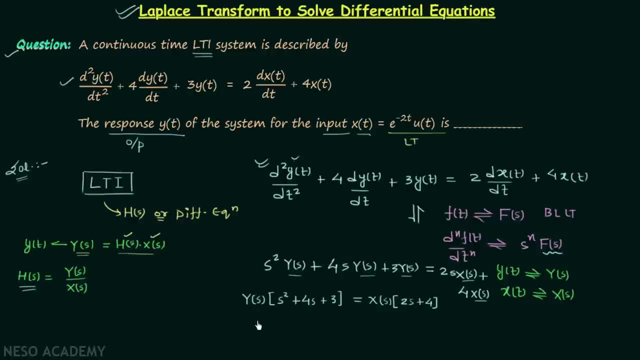 over xs. so what I will do? I will divide both the sides by xs. This will give us ys over xs. So this will give us ys over xs. xs inside the bracket s square plus 4s plus 3, equal to xs over xs inside the bracket 2s. 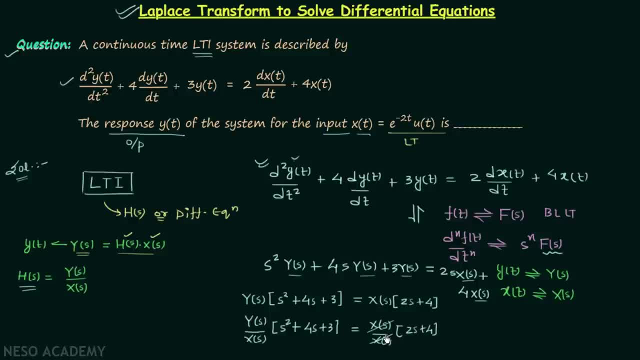 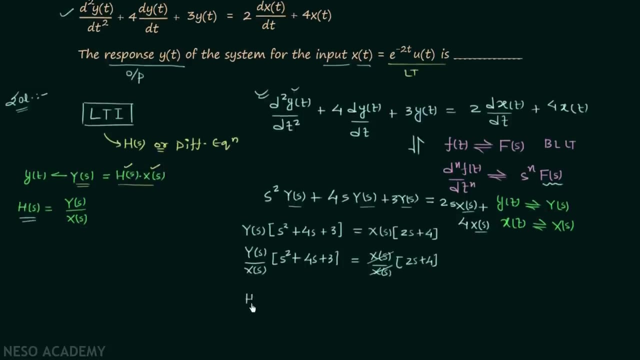 plus 4, xs and xs will cancel out. and now we will divide both the sides by s square plus 4s plus 3, and this will give us ys over xs on the left hand side, and in this way we will have transfer function hs. it is equal to ys over xs and it is equal to 2s plus 4 in. 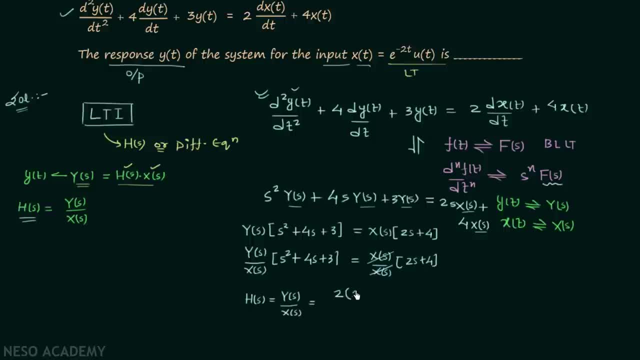 the numerator or I can write 2 inside the bracket s plus 2. I have simply taken 2 common from 2s and 4 in the denominator. we will have s square plus 4s plus 3, or we can write this after the denominator. 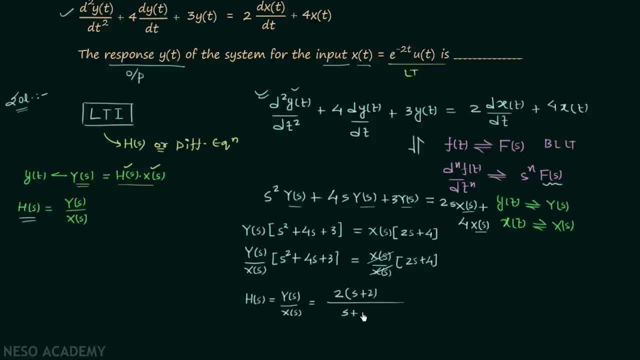 After factorizing, which will give us s plus 1 multiplied to s plus 3, and in this way we have calculated our transfer function, hs, and half of the job is now done. We have calculated hs, and now we will concentrate on calculation of xs. 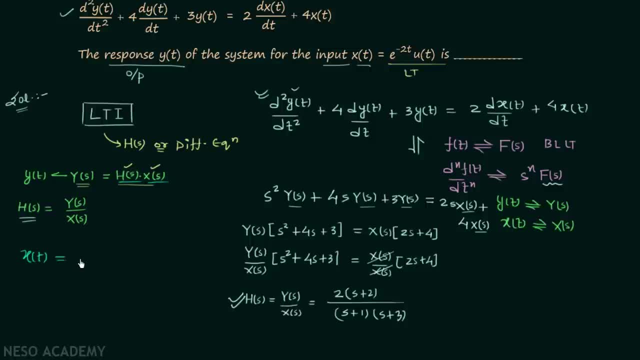 xt, which is the input signal is given in the question. it is equal to e power minus 2t over 2t multiplied to ut and if we take the Laplace transform, we will get xs equal to 1 over s plus 2, and we already know how to obtain the Laplace transform of e power minus 2t multiplied. 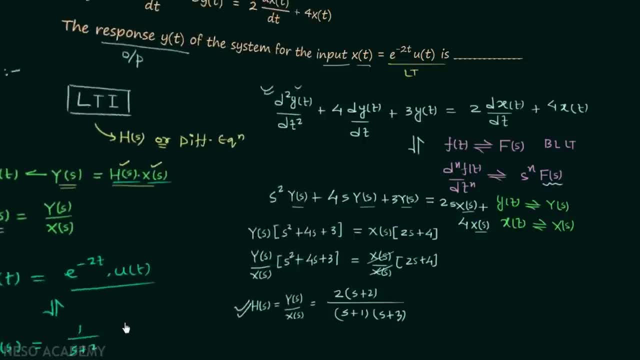 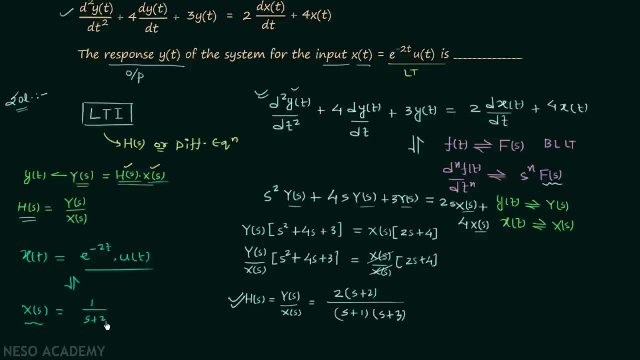 to ut. I am not going to explain it again because we have already done this many times before. so we are getting xs equal to 1 over s plus 2.. And in the next step we will multiply hs and xs. this will give us ys, because ys is. 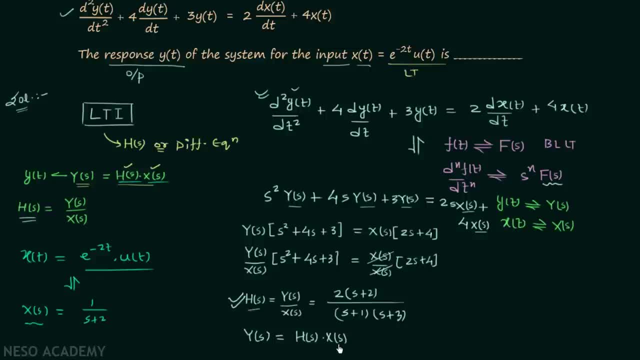 equal to hs multiplied to xs, and after multiplying hs and xs we will have 2 over s plus 1 multiplied to s plus 3, because s plus 2 in numerator of hs will cancel out with s plus 2 in denominator of xs. Now we have ys, it is equal to 2 over s plus 1 multiplied to s plus 3, and we will try to 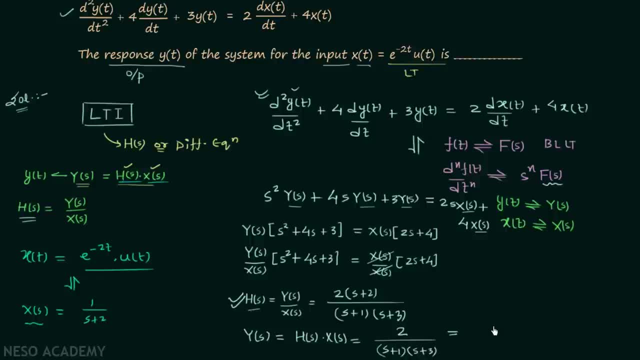 write down this Laplace transform as the combination of standard Laplace transforms using the partial fractions. So, using the partial fraction, we have a over s plus 1 plus b over s plus 3, and we can write this as a multiplied to s plus 3.. 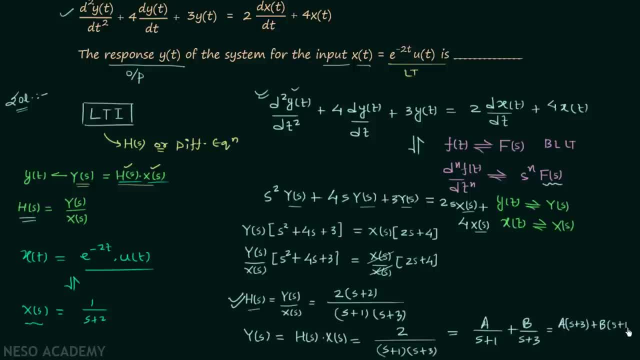 So we have ys equal to 2 over s plus 1 multiplied to s plus 3, and we will try to write down this Laplace transform as the combination of standard Laplace transforms using the partial fractions. So we have ys plus 2 over s plus 2 divided by s plus 1, multiplied to s plus 3.. 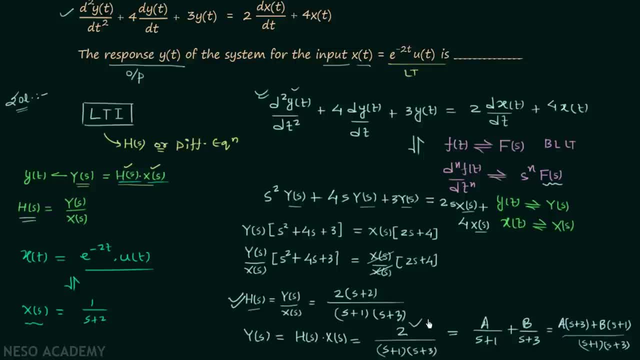 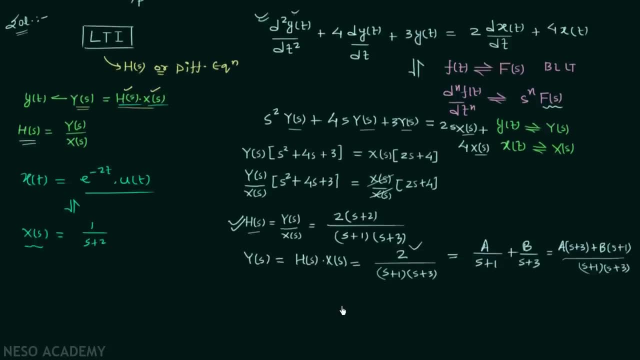 Now compare this with this. you will find 2 is equal to as plus 3 plus bs plus 1.. So in the next step we will write: as plus 3 plus bs plus 1 is equal to 2.. is what we are getting after the comparison. Now we will put s equal to minus 1.. We will 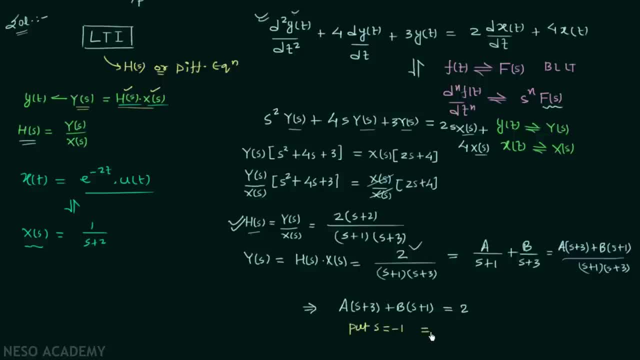 put s equal to minus 1.. This will give us a inside the bracket, minus 1 plus 3 plus b multiplied to 0 is equal to 2.. So from here we are getting: a is equal to 1.. a is equal to 1.. After this, we will put s equal to minus 3.. This will give us a multiplied to 0 plus.